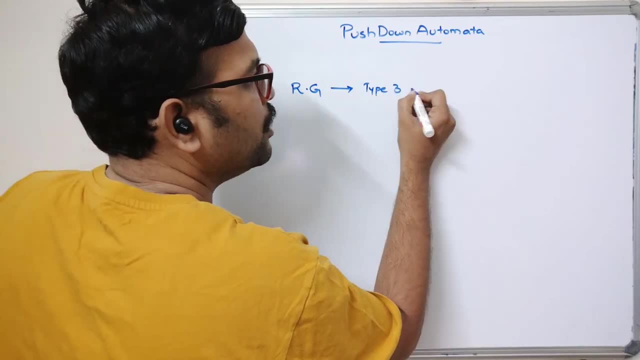 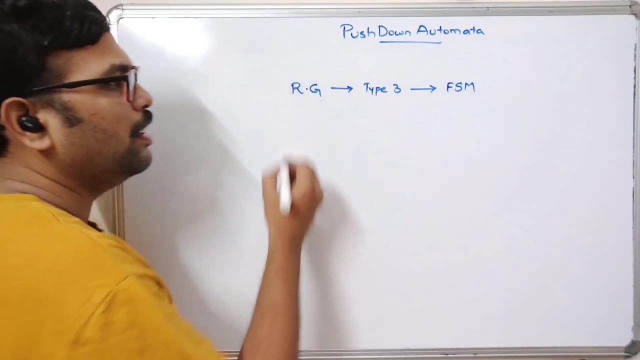 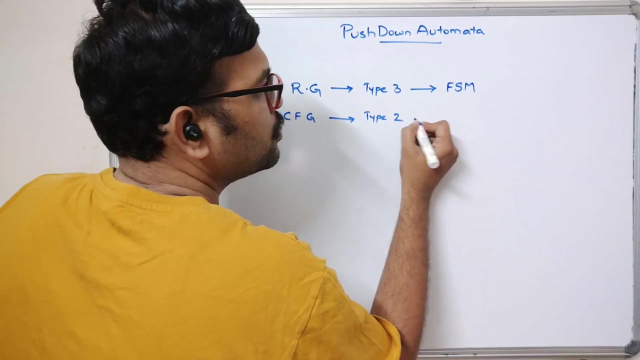 is also called as a type three grammars, And in order to implement these type three grammars, so we required some finite state machines. And now the context free grammar, CFG. these are the type two grammars. So in order to implement these type two grammars, to recognize these grammars, we require push. 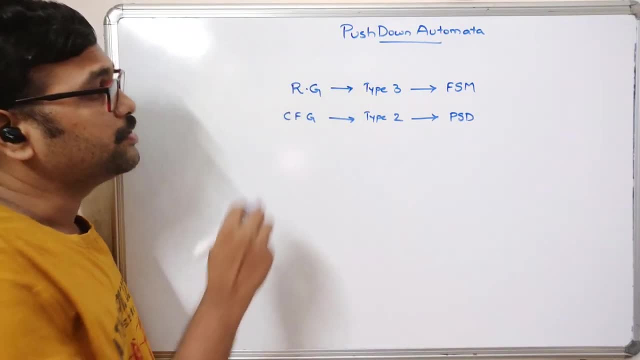 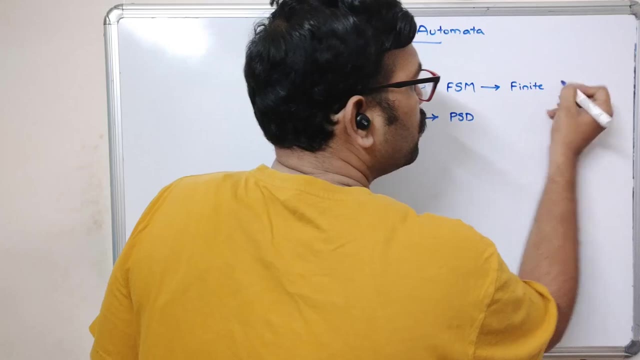 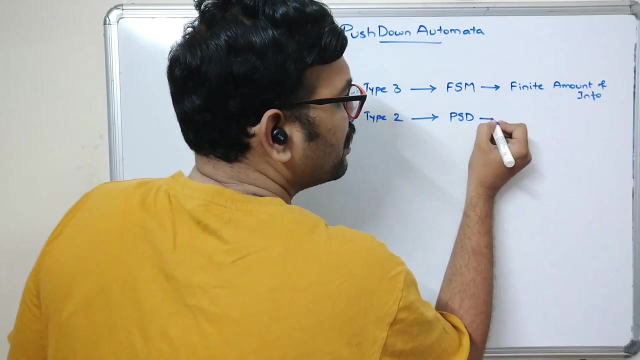 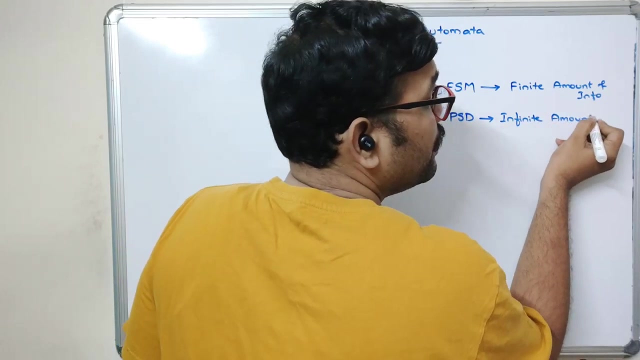 down automata. So what's the difference here? So this type three, these finite state machines, can process the finite state Amount of information. The finite amount of information can be processed here, but here it can process infinite amount of information, infinite amount of information, right So? 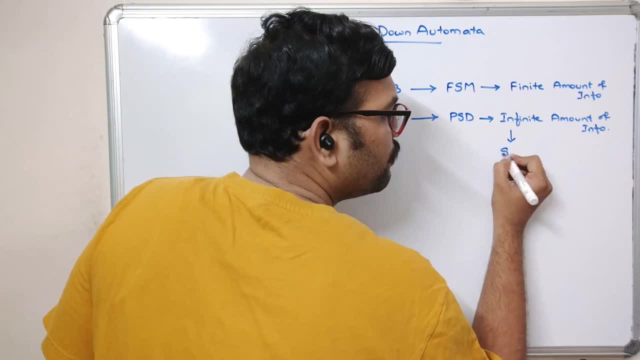 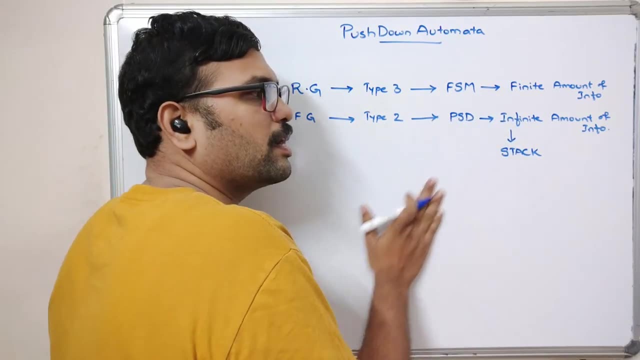 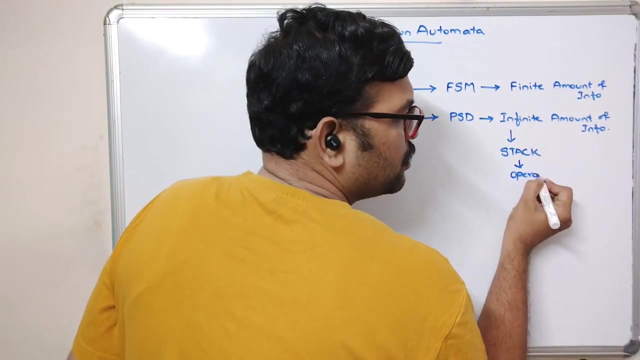 this can be happen with the help of stack, So we'll use some stack, and with the help of the stack, So this push down, automata, process the infinite amount of information and we know that the stack, we are having a different operations, so operations, that is mainly two operations. 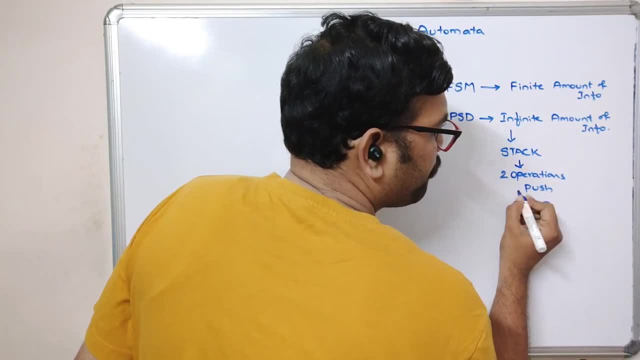 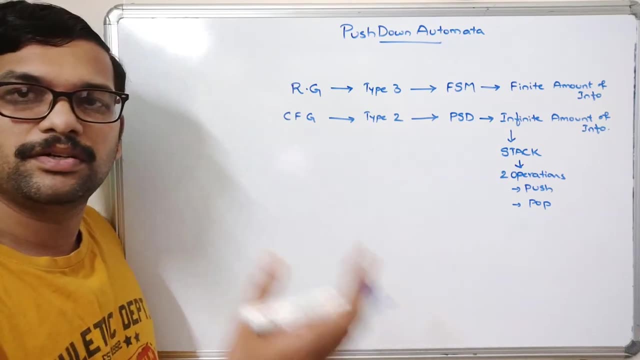 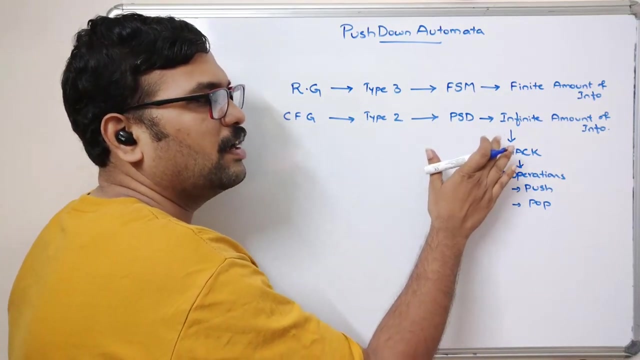 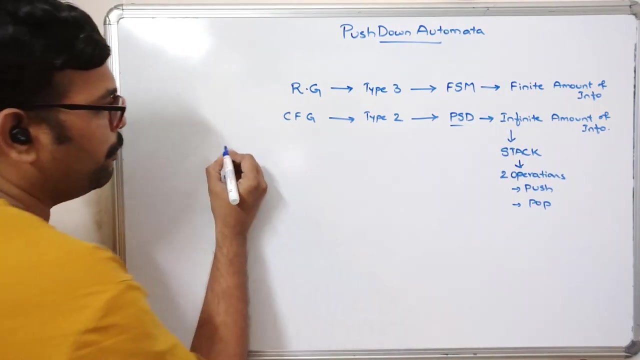 push and pop. so push operation means inserting the element into the stack and a pop is the operation to remove the top of the element in the stack. so we'll do these two operations in the stack and we process the infinite amount of information by the pushdown automata. so there are three components here in the 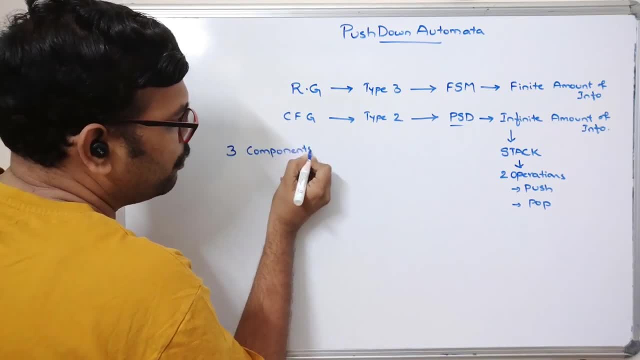 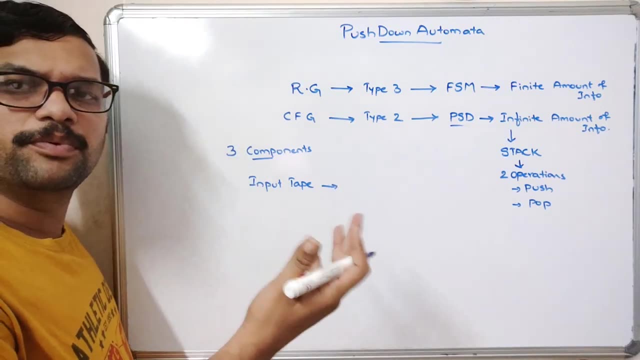 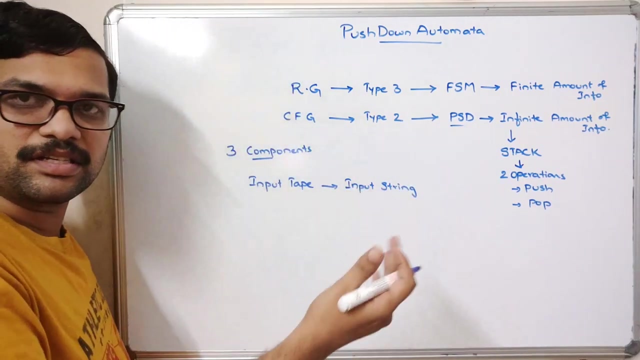 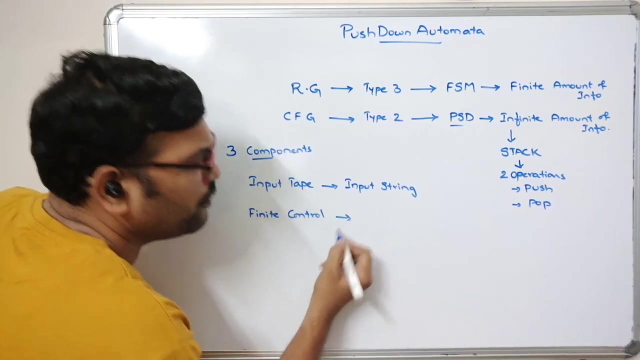 pushdown automata. so what are the three components? the first one is input tape, so input tape. so input tape is nothing but our input string, okay, so that is nothing but input string which has to be processed, okay. and the next one is finite control, so which will perform the push and pop operations. push and pop operations in. 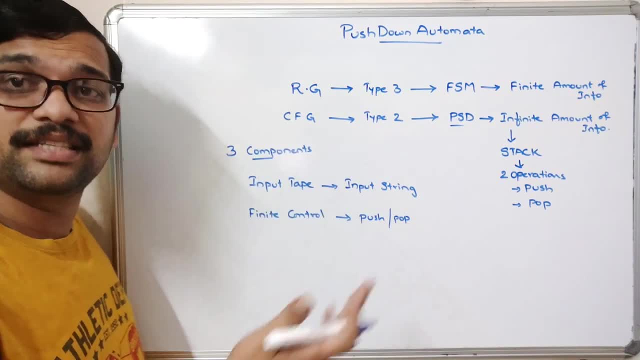 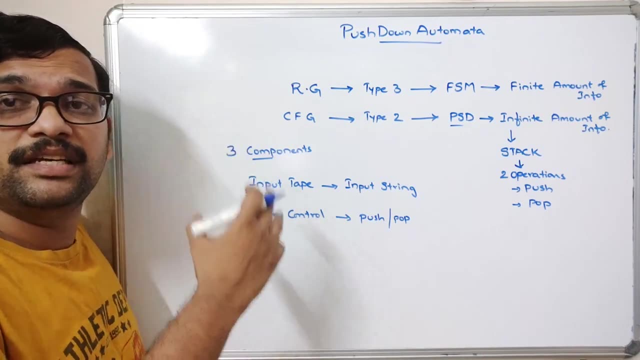 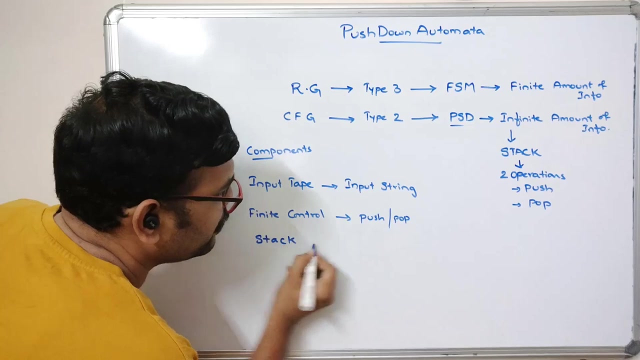 order to process the information, in order to change the states- okay, so we know that. so if they, for every input, the state can be changed from one to another, so that process can be done by this finite control. and the third component is a stack in order to maintain the elements. the elements will be maintained. 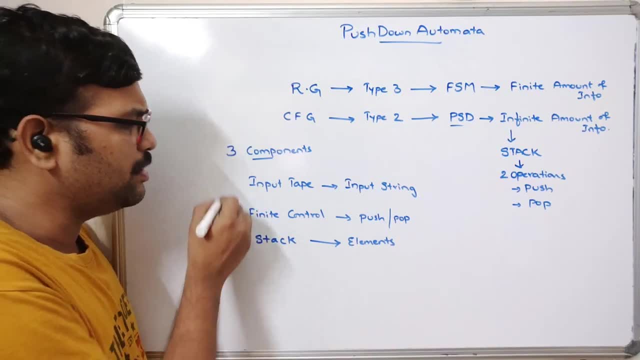 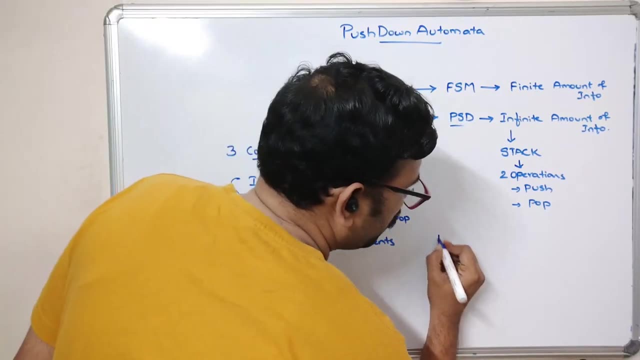 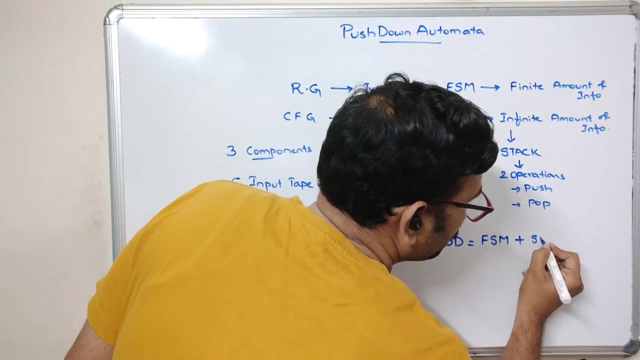 in this stack, right? so these are the mainly three components which are available in this pushdown automata, and see pushdown automata can also be called as the finite state machine plus stack. so all the rest of the things are same. all the rest of the things are same, but only the difference. 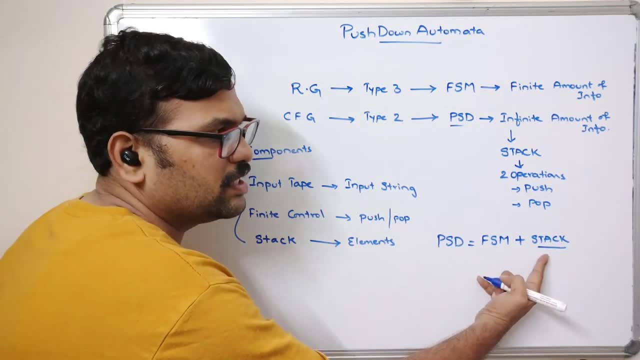 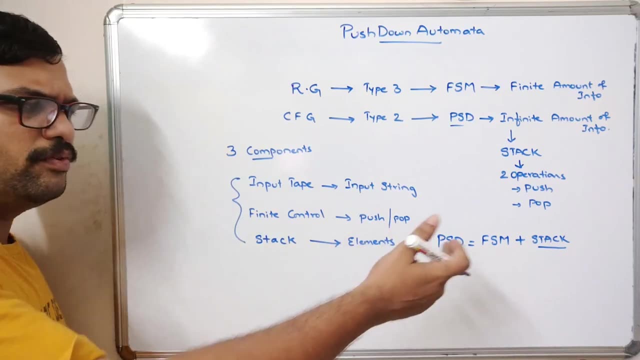 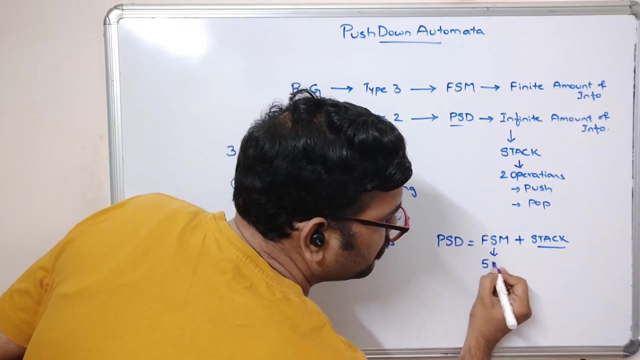 is the stack, so by using this stack it will process the infinite amount of information right now we can. so we have discussed about the definition of finite state machine in the previous sessions. right, so finite state machine can be represented as a five tuple: right and plus so two. 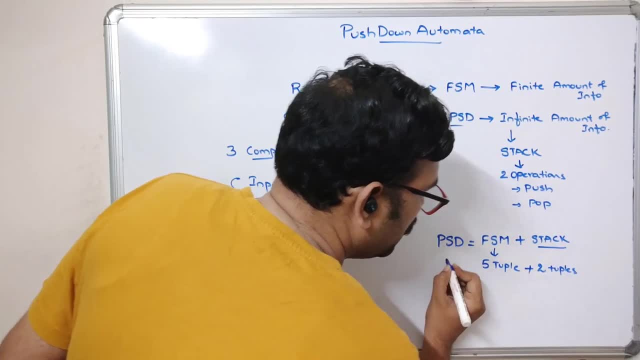 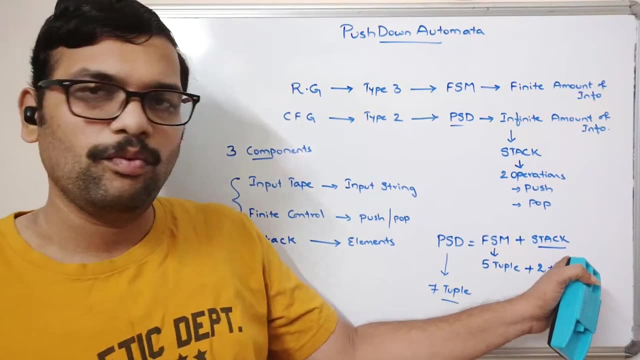 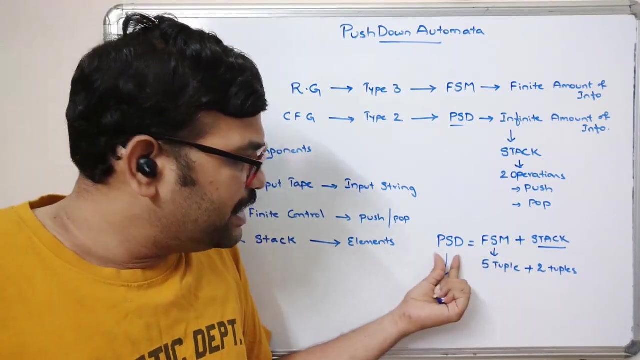 more tuples will be added so the psd can be represented as seven tuple. so two tuples for a stack, one is for scoring the stack symbols and another one is for the top of the stack. okay, so stack. So PSD, that is a push down automata- can be defined as a 7 tuple. The 5 tuple is common. 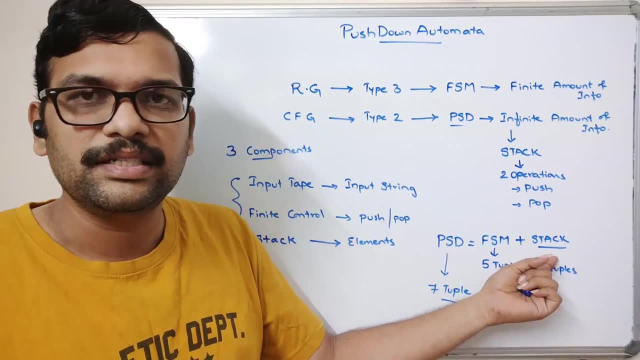 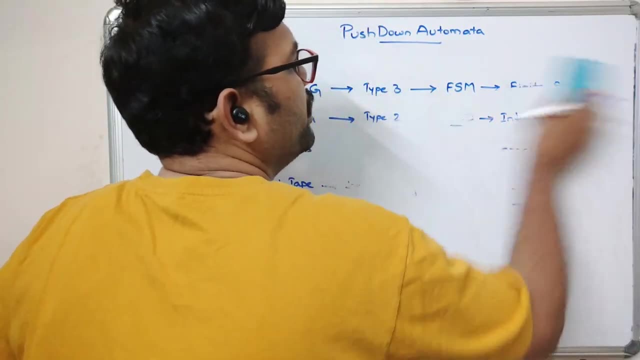 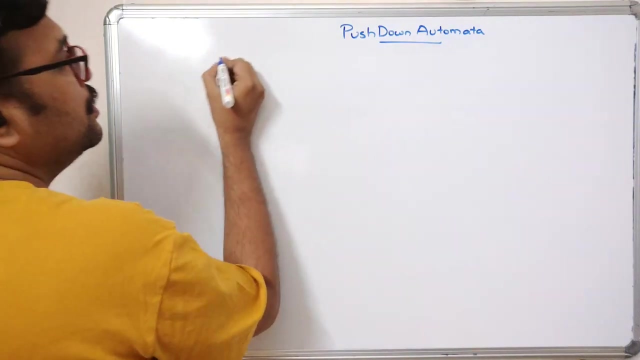 with the finite state machine and the 2 tuples are for the stack related to the stack. Now we will see the definition of PSD. that is a push down automata. We will see the definition of push down automata. So push down automata, see the name itself indicates push and down. that is a. 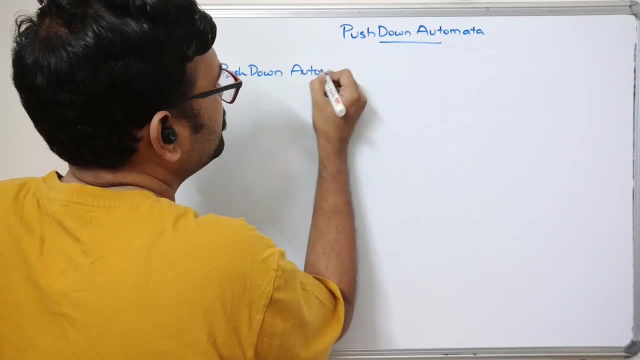 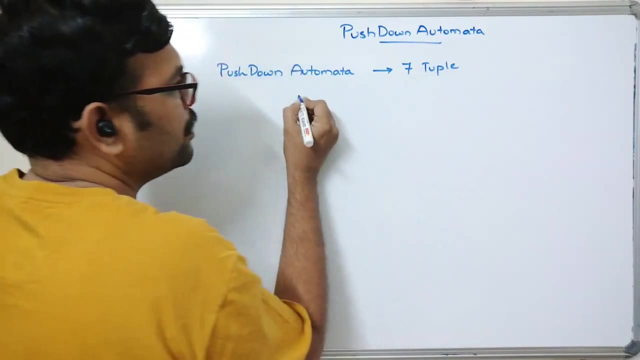 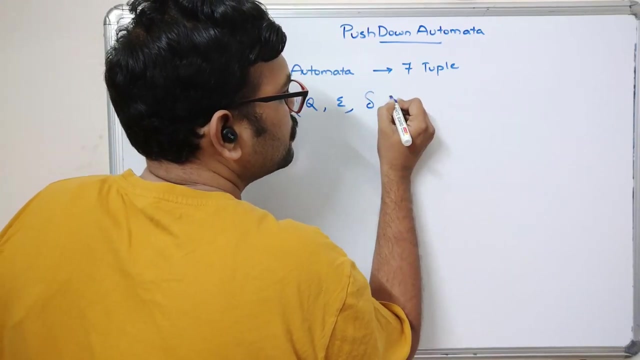 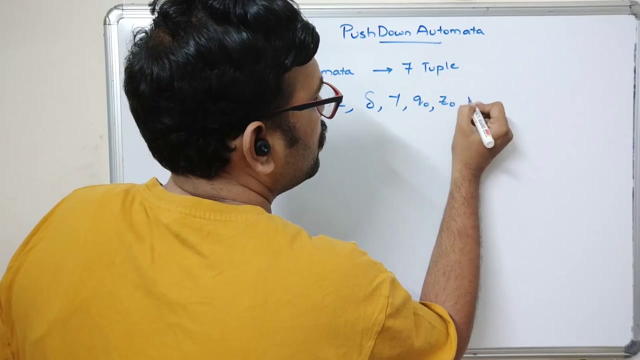 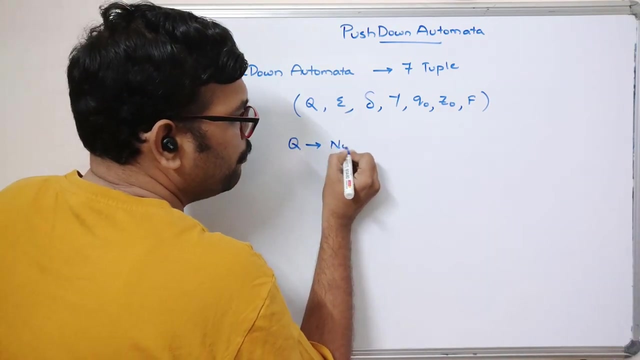 push and pop right, Push down. automata can be defined as 7 tuple. So first one is a Q sigma function, gamma gamma, Q0, Z0, F, Q0, Z0 and F. So you can see here Q is the number of states. So that is common. 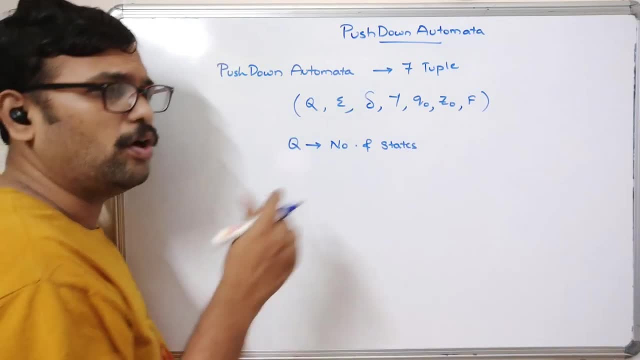 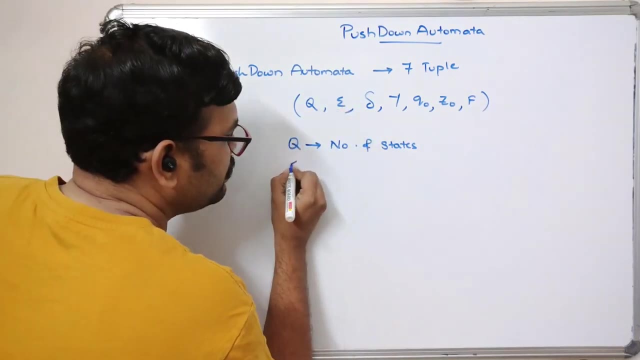 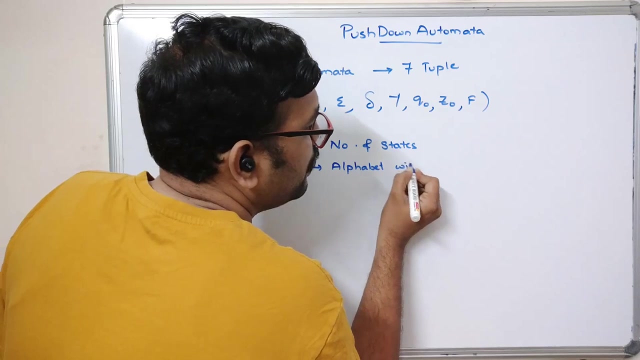 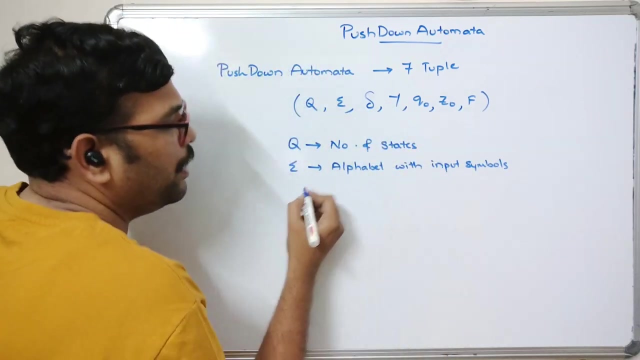 which we have discussed. in the finite state machines, All the states can be represented in a set of finite number of states, is represented in Q And sigma is alphabet, Alphabet with input symbols, So there will be different symbols And delta is a transition. 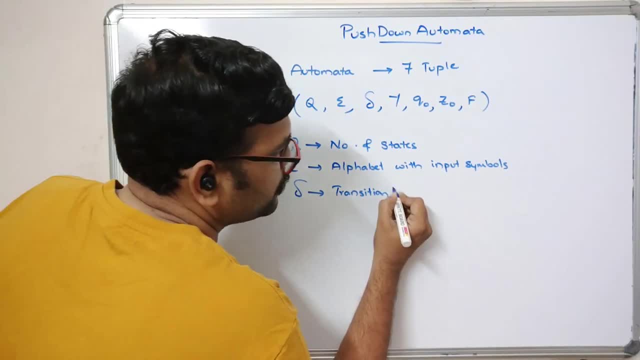 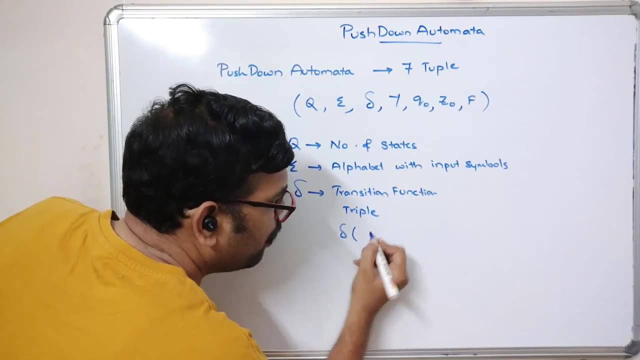 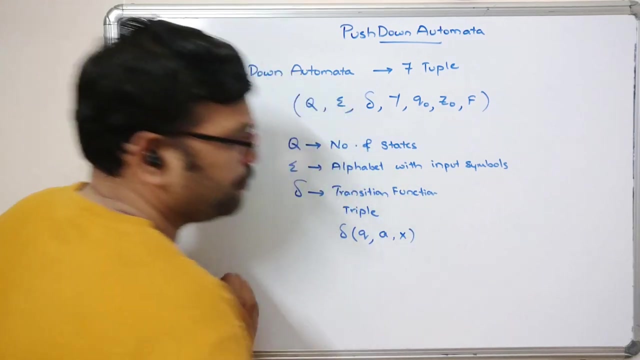 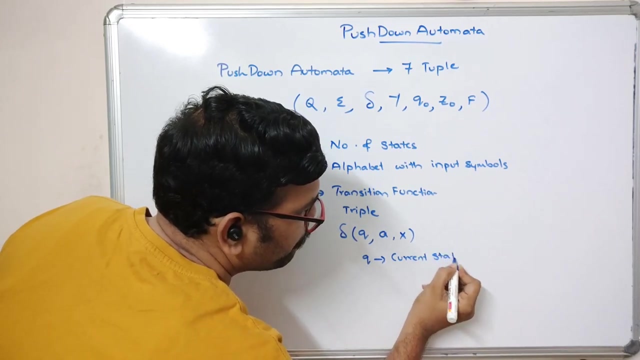 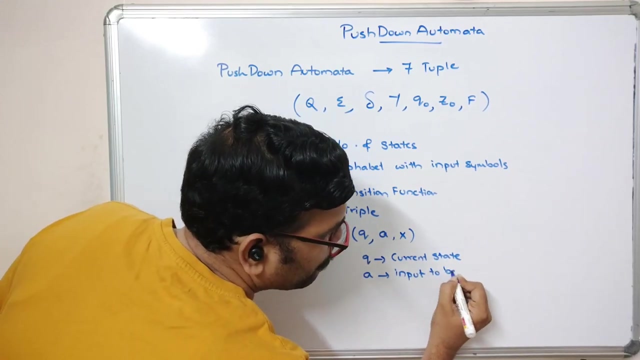 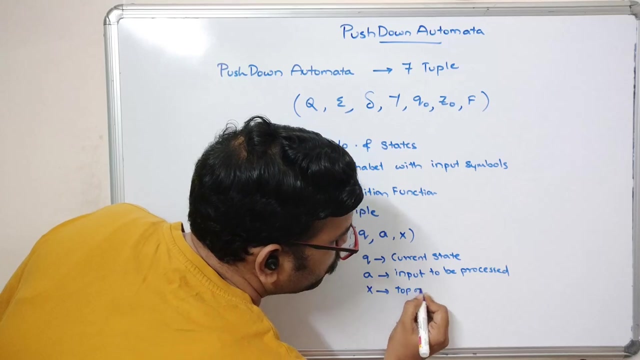 function, Transition function, And this transition function is represented as a triple. That means delta of Q- Okay Okay. A- and X, Where Q is a current state And A is input to be processed. X is a top of a stack. X is a top of a stack. 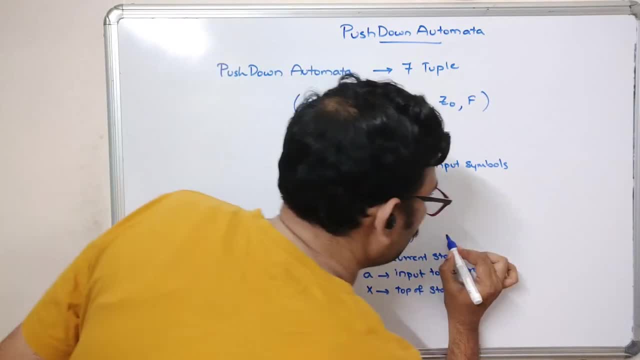 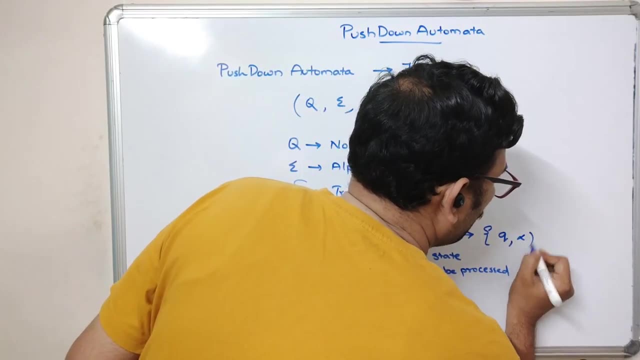 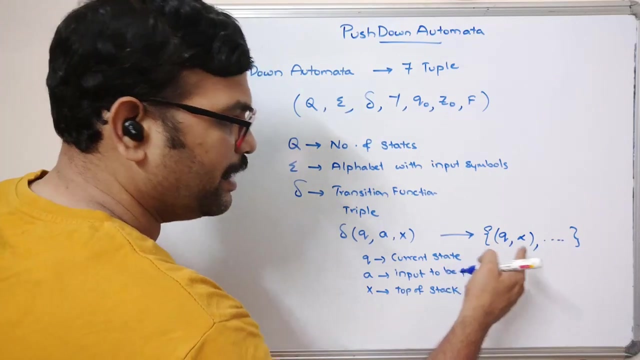 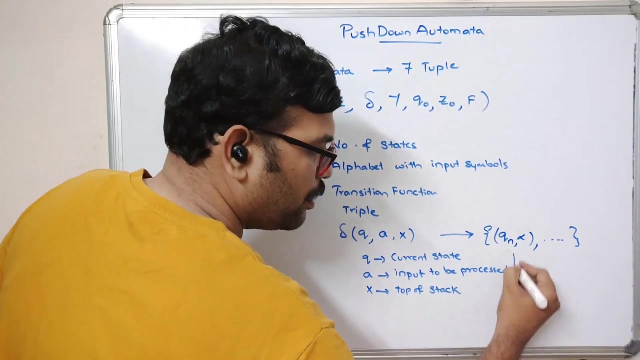 Okay, Okay, Okay. And the result of this transition will give a finite pace, that is a Q, and some alpha, A finite pace of sets, that is a Q and alpha. And here we will go with Qn, Okay, Qn, So where Qn is a new state. 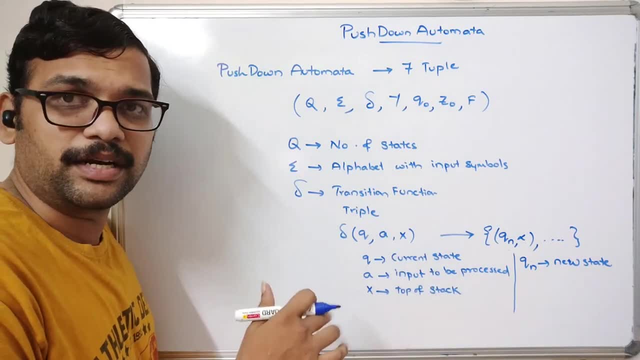 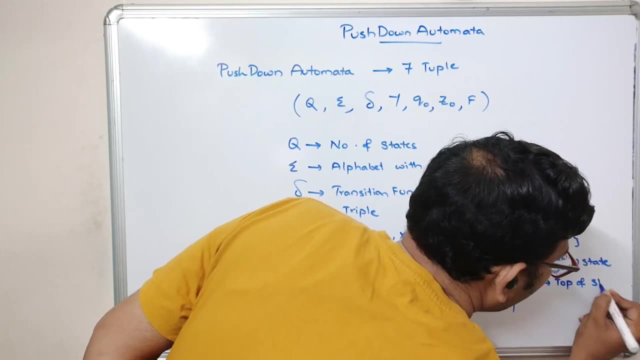 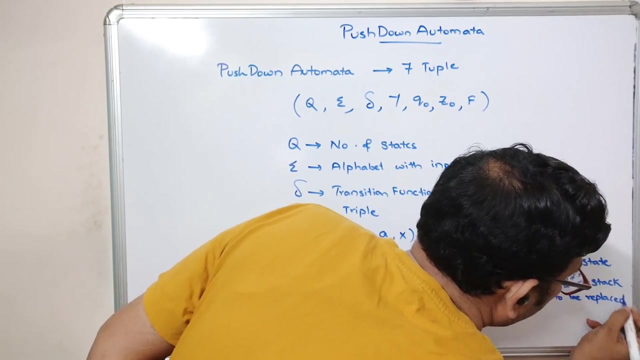 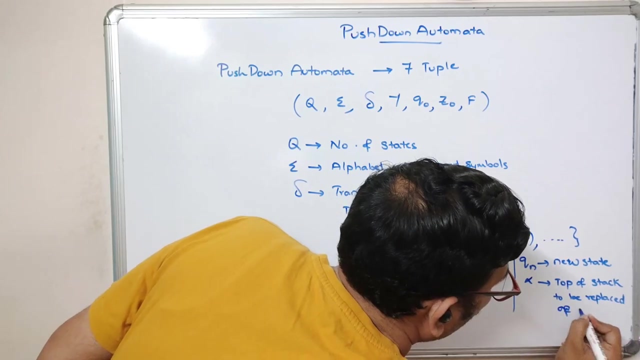 So sometimes it may be that it remains in the same state, Right? So, whatever it may be, Qn is a new state And alpha is a top of stack to be replaced. Okay, So previously X is a top of the stack, Now X will be replaced. 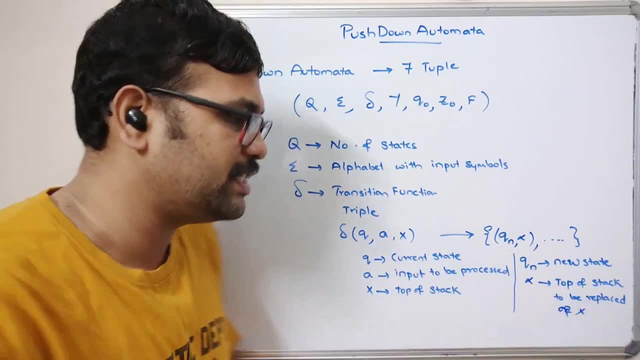 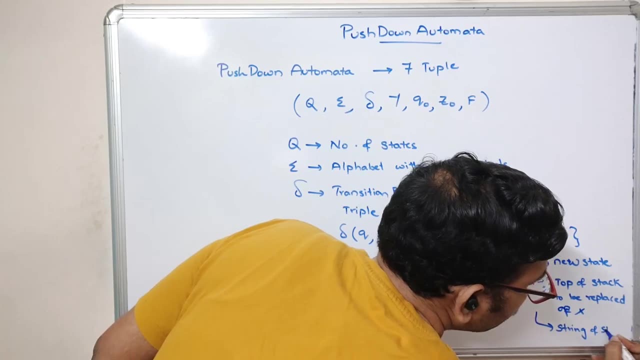 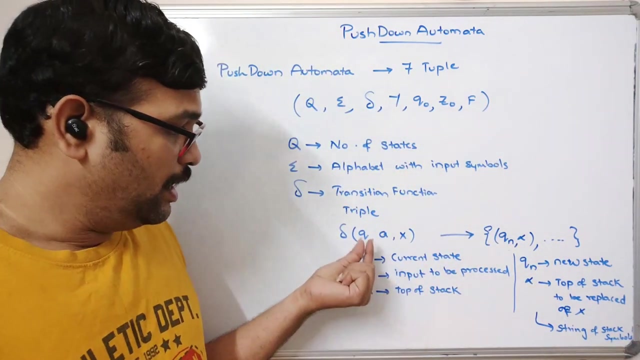 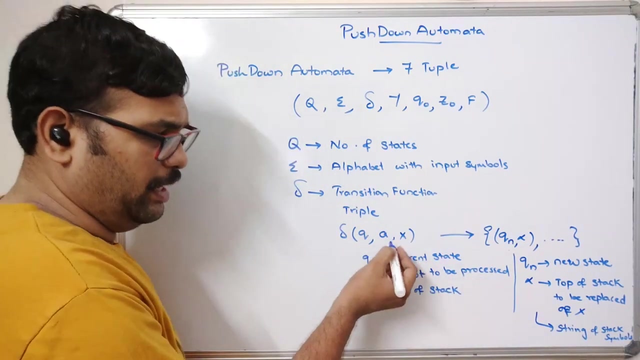 So alpha can be a top of a stack And alpha can be a string of stack symbols, A string of stack symbols. So Q is a current state, A will be the input to be processed And X will be the top of the stack And, based upon the input, we can change the state with a new top of the stack. 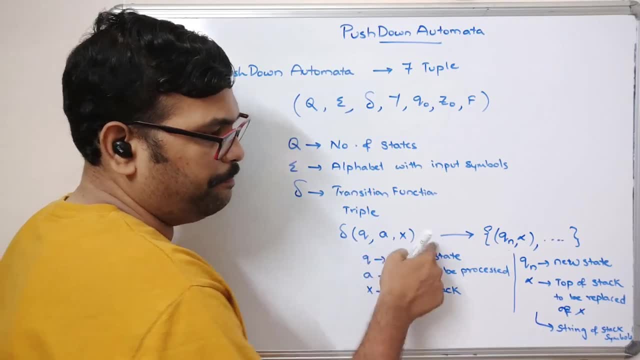 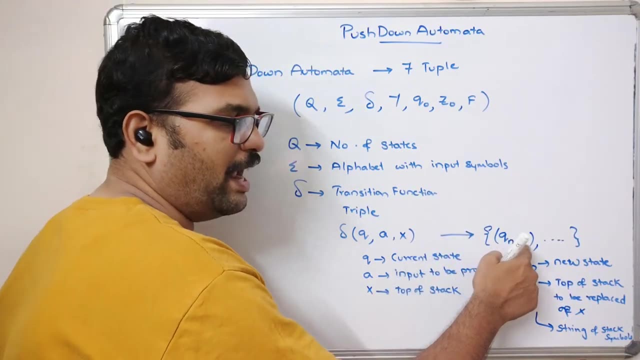 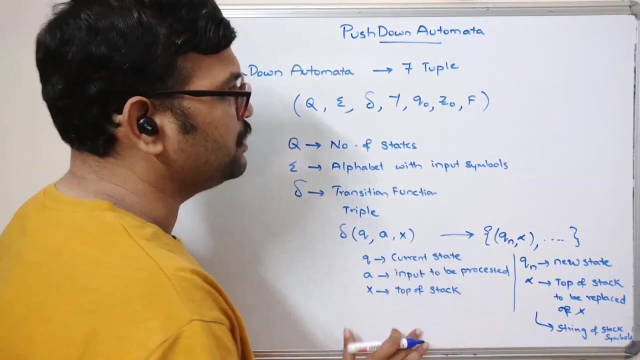 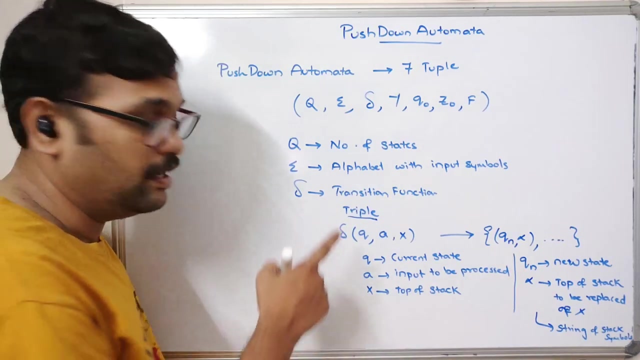 Okay, So this may be. this transition function will give a pair of sets with a new state and the new top of the stack. So if you take an example, you will be understanding. So this is a transition function in this particular push down automata. Okay, It will be represented as a triple. It will be represented as a triple And the next one is a gamma. 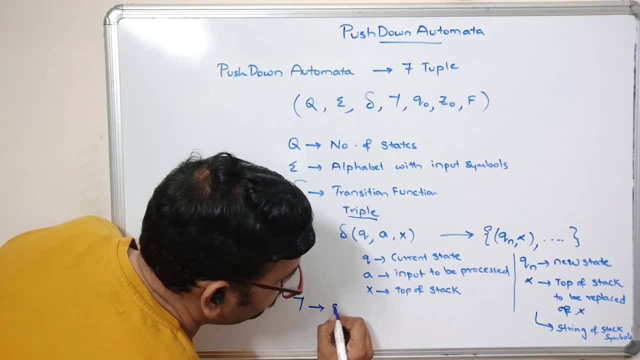 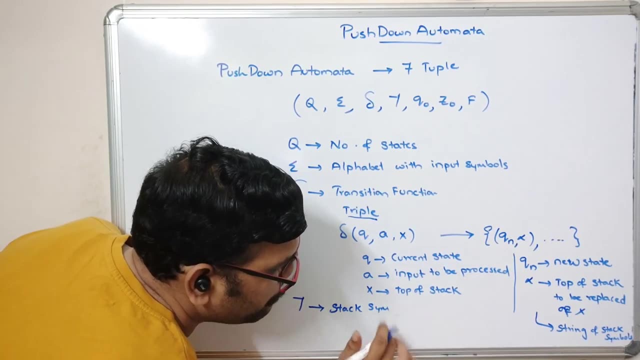 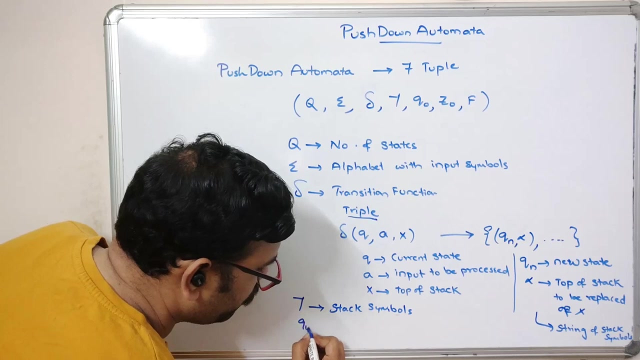 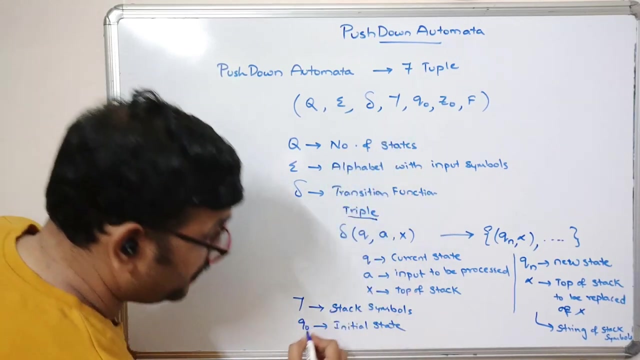 Which is nothing but stack symbols. so, whatever the symbols we are going to push and pop from the stack, all those things, you should be represented in a gamma stack symbols. and we know that the q naught is a initial state- here also the same thing, initial state. and a z naught- a new thing, z naught. 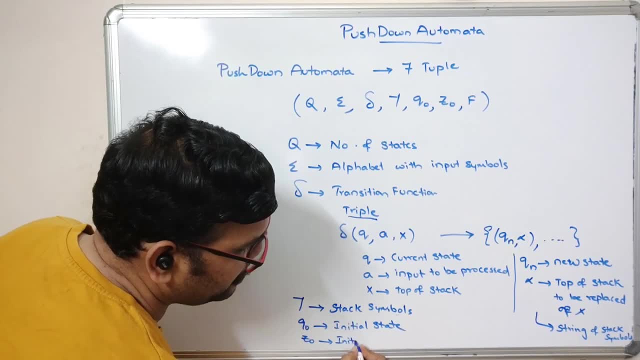 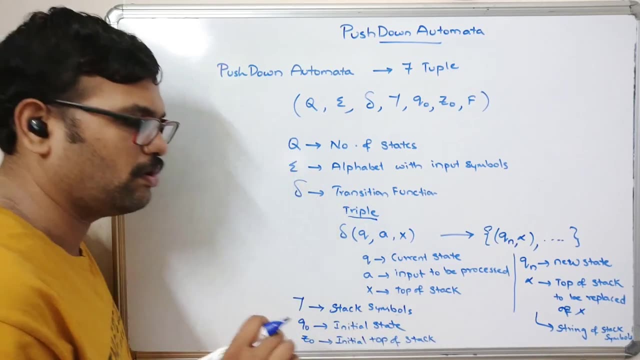 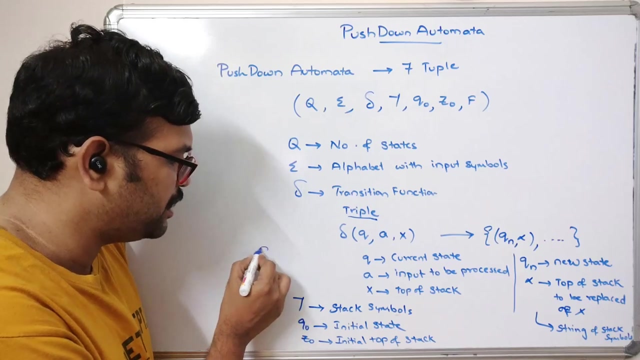 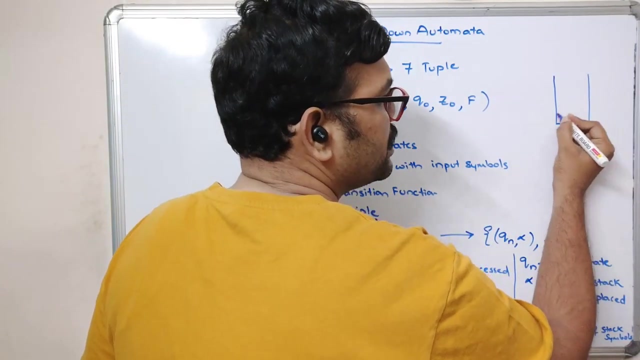 is a initial top of stack. so, before processing any sort of input, the initial top of the stack will be z naught. okay, so in some cases you can be represented as dollar or hash, whatever it may be, the in the by default. by default, the top of the stack will be z naught, so this will be the top. 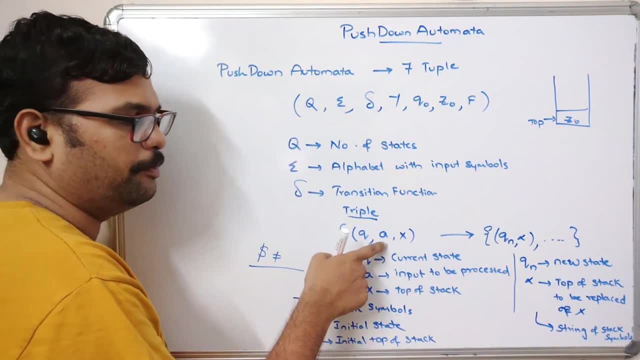 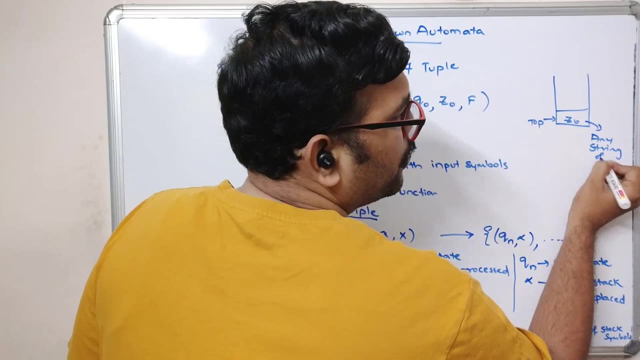 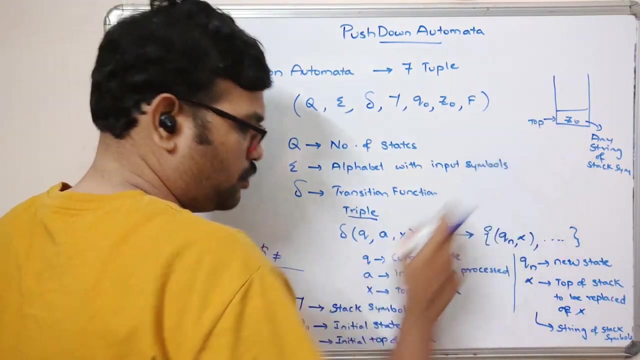 of the stack. so, based upon the pattern of the stack we are going to be representing, z naught transition function, the state and input. this z naught can be replaced with any string of stack symbols, any string of stack symbols, right, but initially the top of the stack will be z. 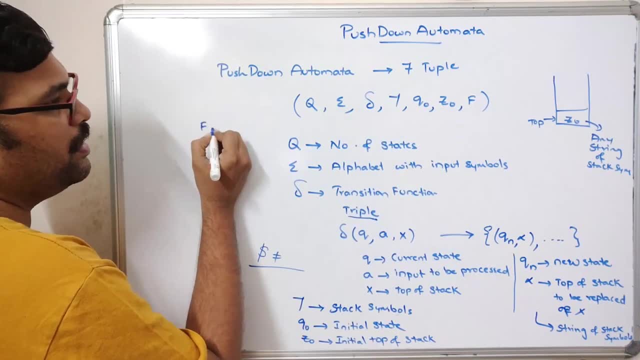 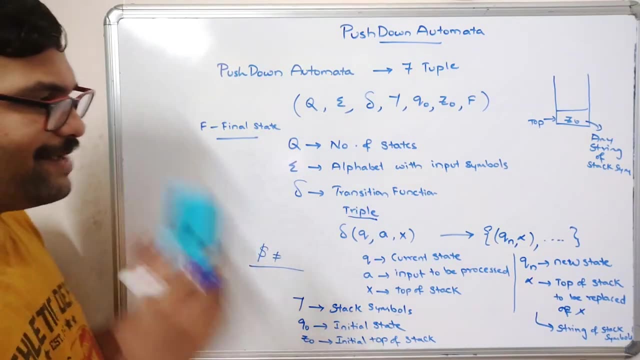 naught, so that z naught here. and finally, f. f is a final state. we know that f will be the final state. so this is the seven tuple that the pushdown auto function will be the final state. so this is the seven tuple that the pushdown auto. 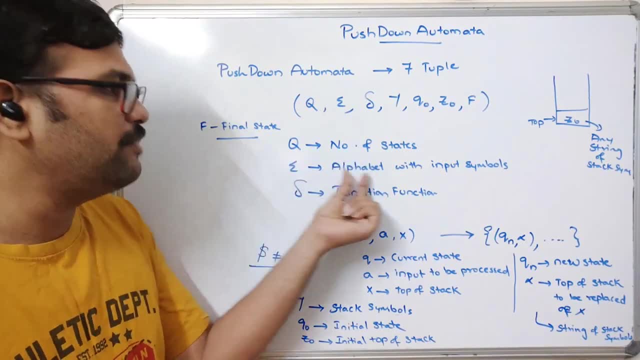 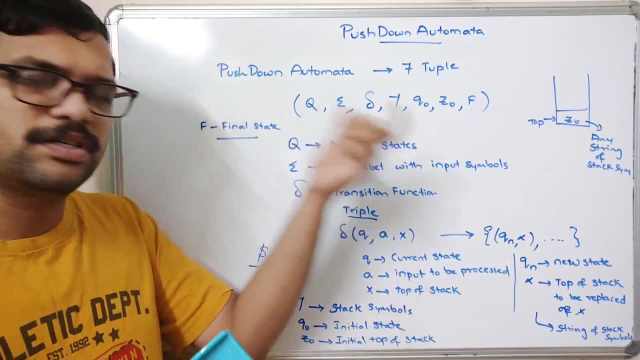 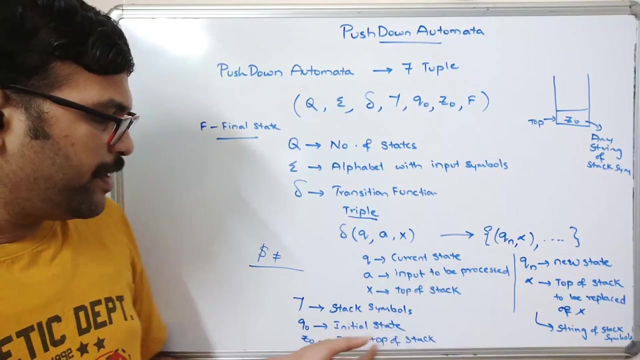 can be defined so: q, the number of states, sigma, alphabet, with the input symbols. delta is a transition function which is similar to our transition function in the finite state machines, but here we represented in a triple so, and the result will be with a pair of sets and gamma, with 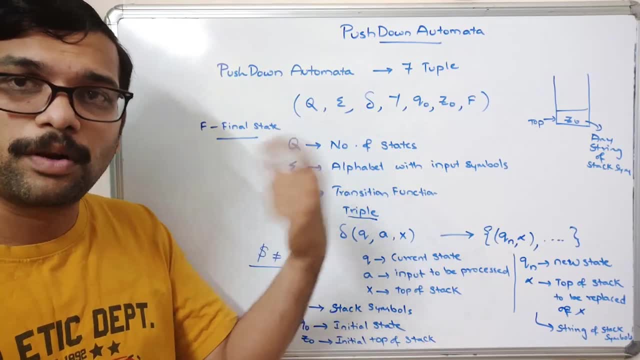 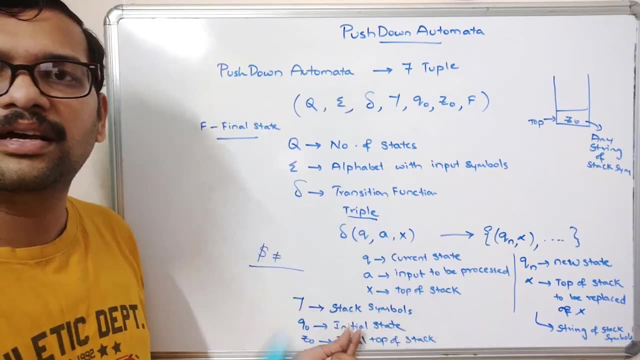 this tag symbols. so whatever the symbols we are going to push or a pop from the stack, so those tag symbols will be represented in a gamma. and q naught is the initial state we know that we have seen in the final state machines and z naught is an initial top of the stack and f will be the final state.